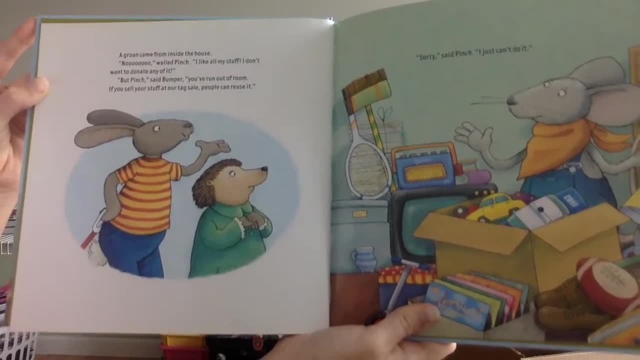 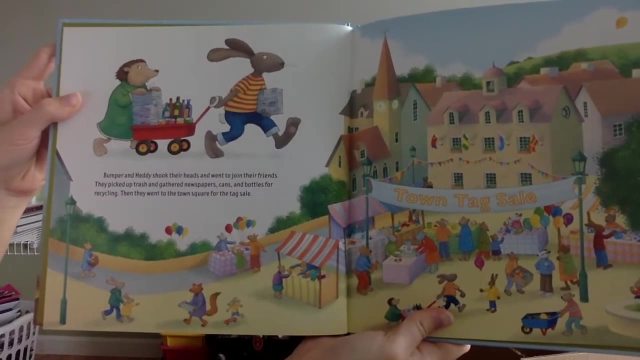 tag sale. people can reuse it. Sorry said Pinch, I just can't do it. Bumper and Hetty shook their heads. They were so excited. They were so excited. They shook their heads and went to join their friends. They picked up trash and gathered. 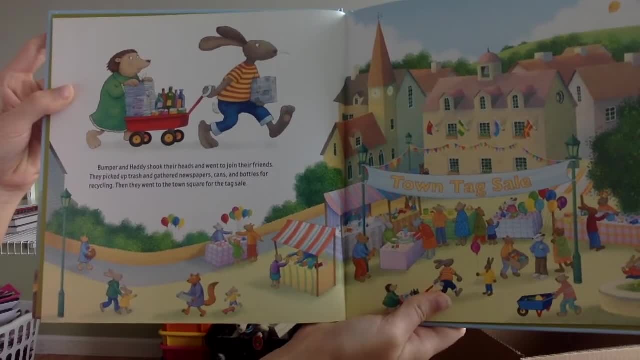 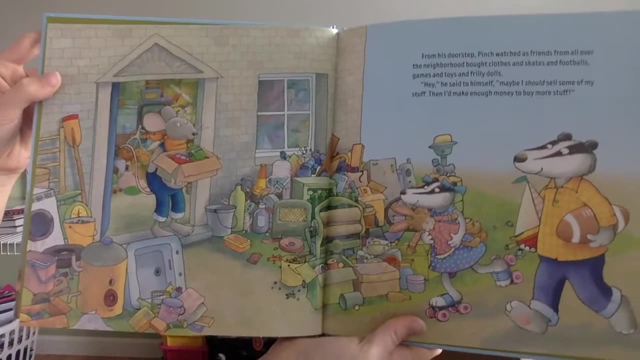 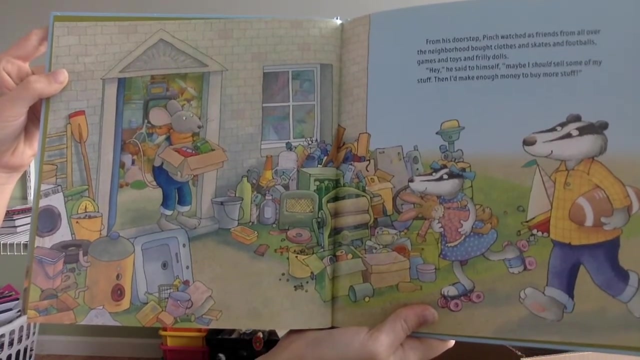 newspapers, cans and bottles for recycling. Then they went to the town square for the tag sale. From his doorstep, Pinch watched as friends from all over the neighborhood bought clothes and skates and footballs, games and toys and frilly dolls. 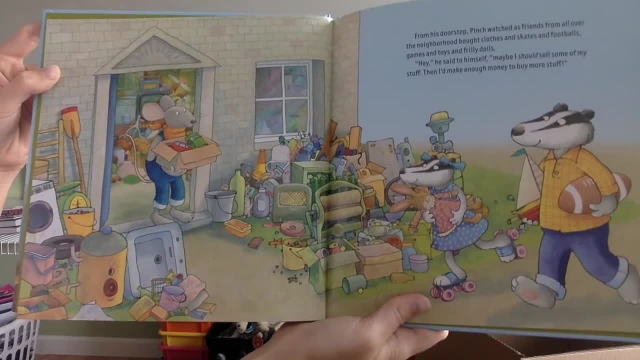 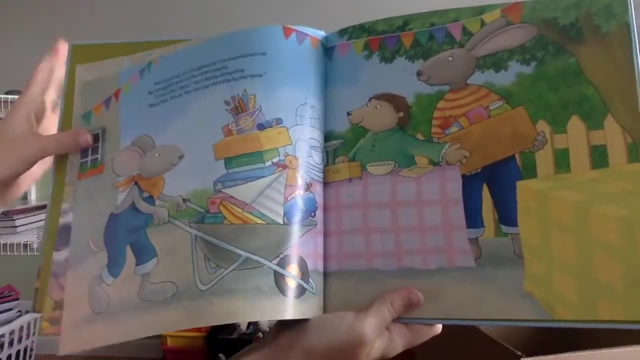 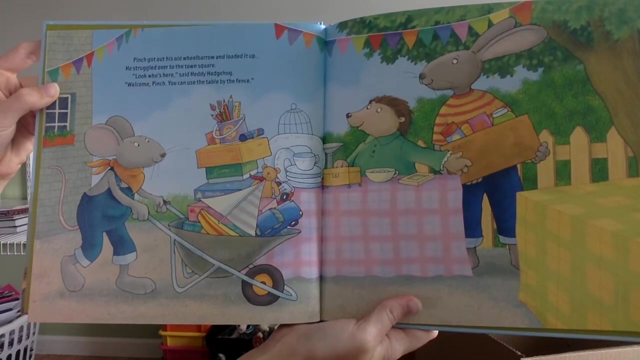 Hey, he said to himself, maybe I should sell some of my stuff, Then I'd make enough money to buy more stuff. Pinch got out his old wheelbarrow and loaded it up. He struggled over to the town square. Look who's here, said Hetty Hedgehog. Welcome Pinch. You can use the table by the fence. 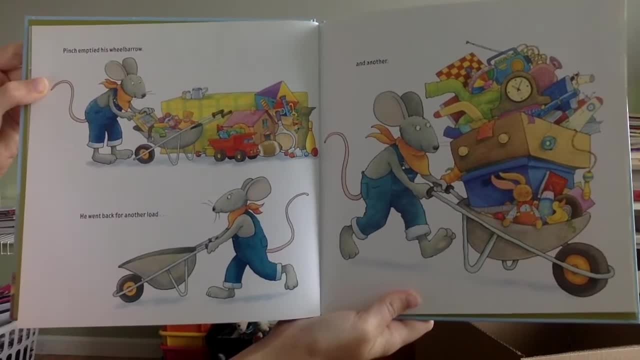 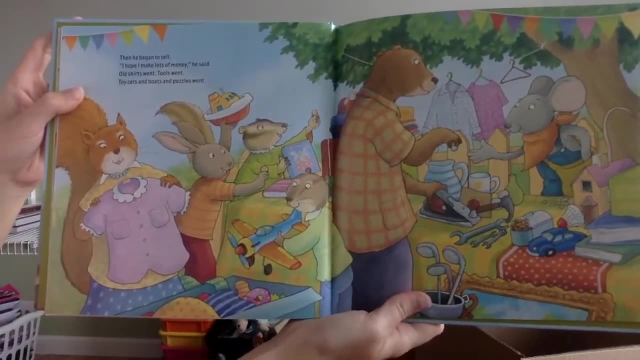 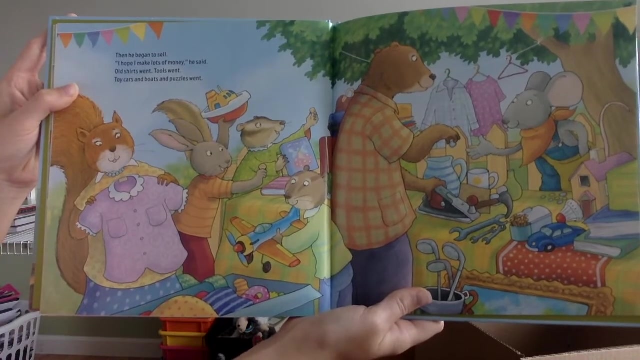 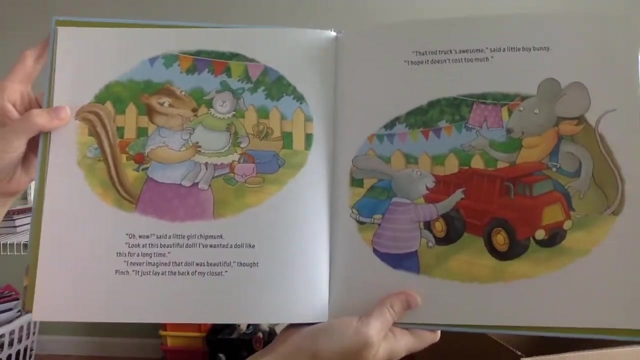 Pinch emptied his wheelbarrow He went back for another load and another. Then he began to sell. I hope I make lots of money, he said. Old shirts went, tools went, toy cars and boats and puzzles went. Oh wow, said a little girl chipmunk, Look at this beautiful doll. I've wanted a doll like this for a long time. 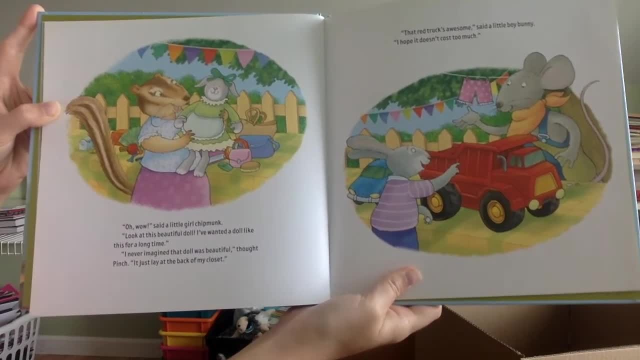 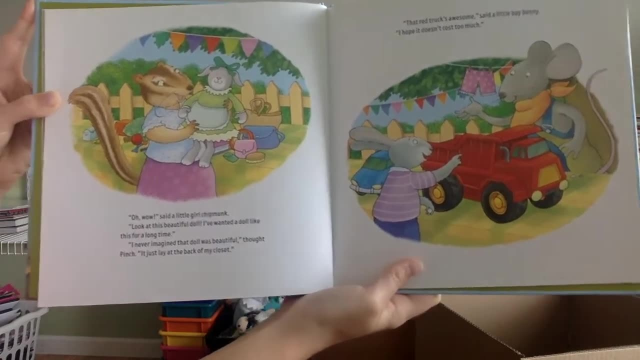 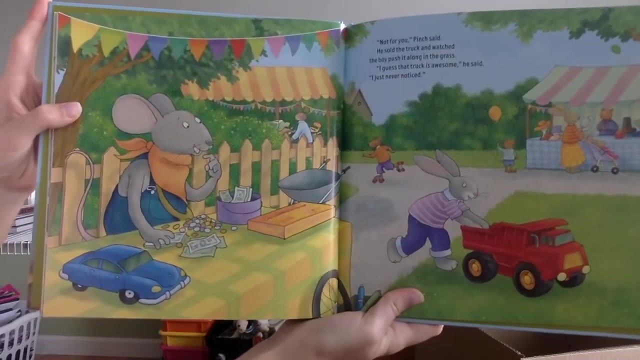 I never imagined that doll was beautiful, thought Pinch. It just lay at the back of my closet. That red truck's awesome, said a little boy, bunny. I hope it doesn't cost too much- Not for you, said Pinch. 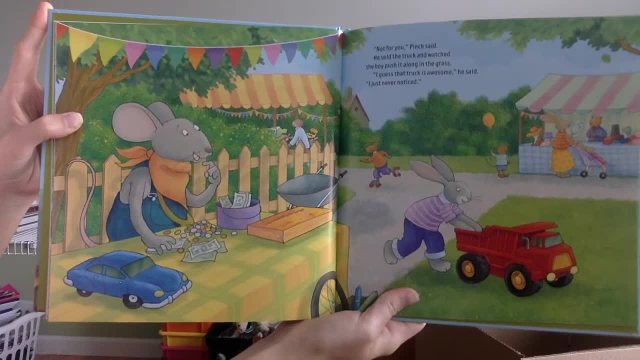 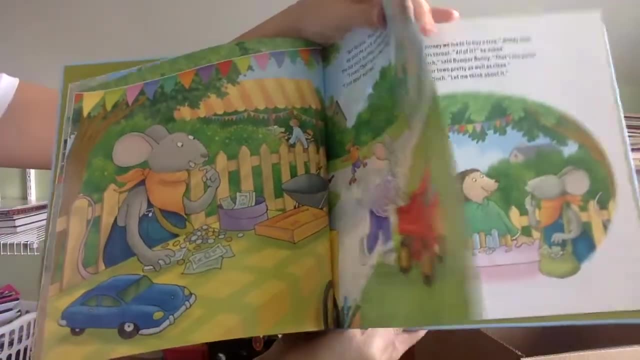 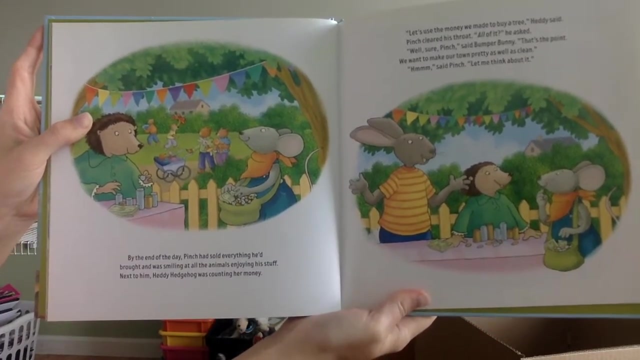 He sold the truck and watched the boy push it along in the grass. I guess that truck is awesome. he said I just never noticed. I just never noticed had sold everything he'd brought and was smiling at all the animals enjoying his stuff Next to him. 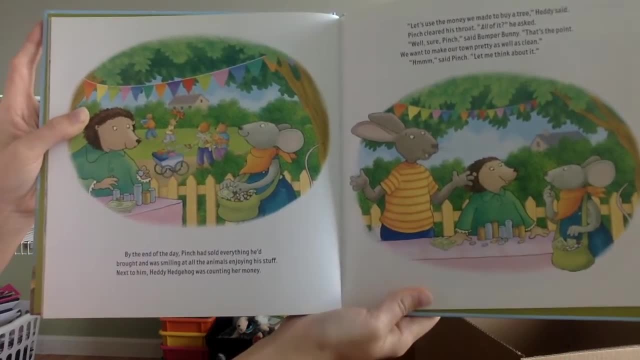 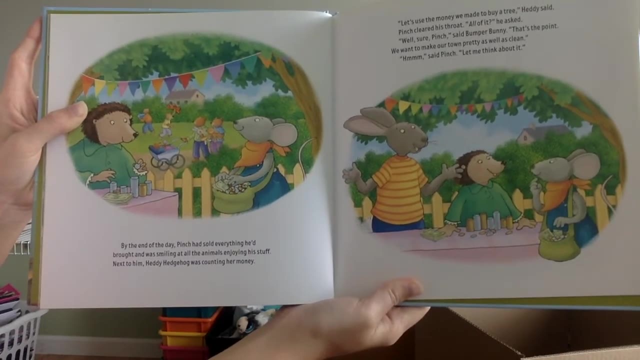 Petty Hedgehog was counting her money. Let's use the money we made to buy a tree, Hetty said. Pinch cleared his throat All of it. he asked. Well, sure, Pinch said Bumper Bunny. That's the point.